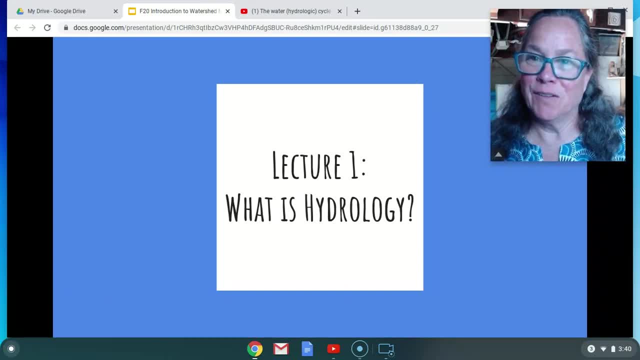 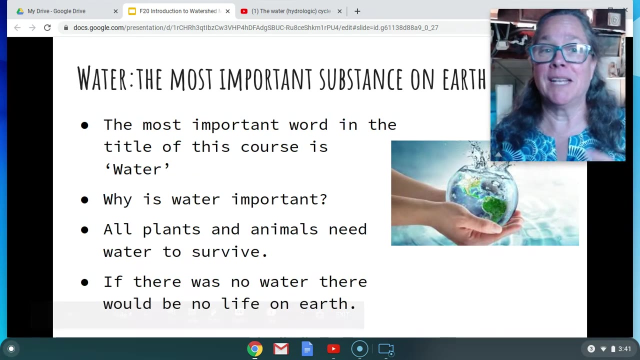 Hey there and welcome to our first lecture in this module, the introduction to hydrology and watershed management. So we're going to answer the question: what is hydrology? But before I talk about that, I'd like to talk a little bit about water, because it is the 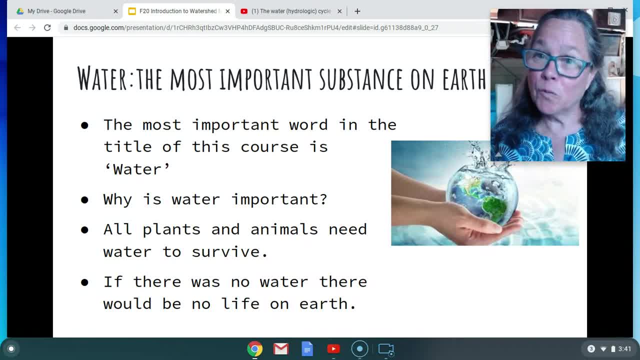 most important substance on Earth and the most important word in the title of this course: water. Why is it important? Life is not possible without water on this Earth. We can't survive without water, and I think you guys can think about that. So this is going to be an important 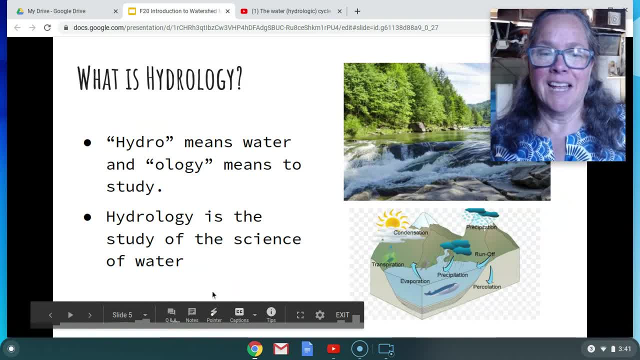 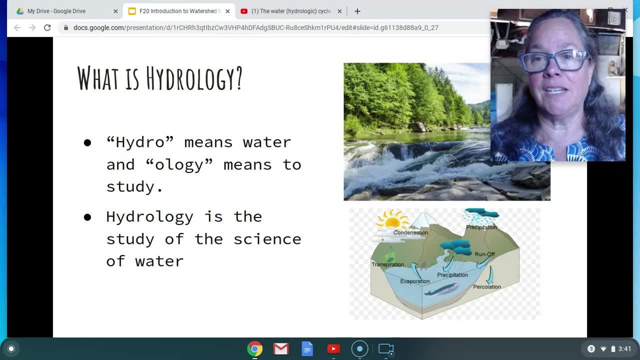 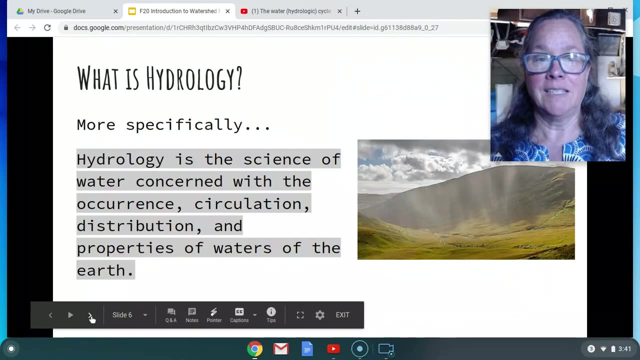 topic in this class. So hydrology, what is hydrology? Well, hydro means water and ology means to study. Hydrology is described as the study of the science of water, and in a moment I'm going to give you a more detailed definition. So, more specifically, hydrology is the science. 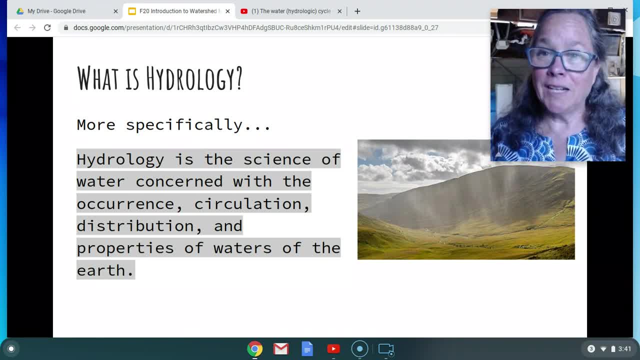 concerned with the occurrence circulation, distribution and properties of water on Earth. This is important. We're going to be talking in a few weeks about those properties of water and then we're going to be talking through this whole course about the occurrence circulation. 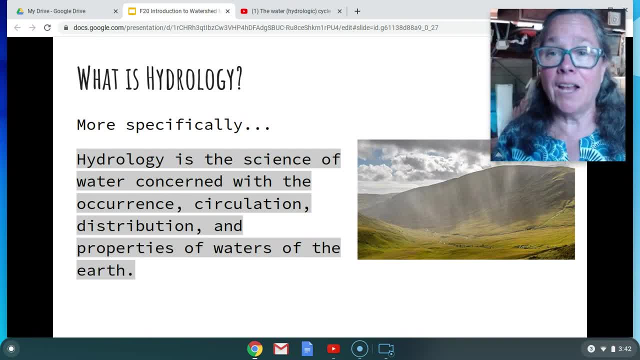 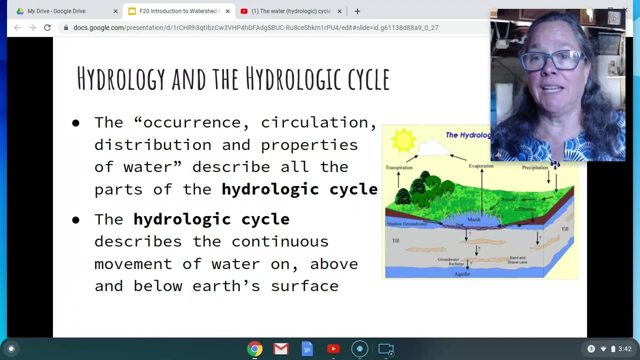 and distribution of water And how that hydrology- the study of hydrology or the science of water- fits into watershed management. So hydrology is really talking about the hydrologic cycle, because the hydrologic cycle is looking at the occurrence where water comes from, the circulation, how it moves around. 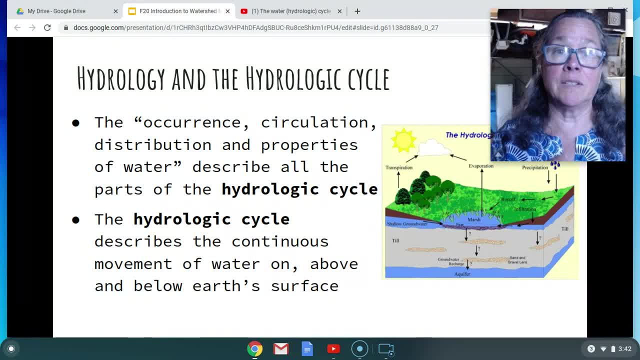 and the distribution. Where is it- Where is it on the Earth, Where is it in the watershed? And the properties of water that make it move from one form of matter to another. these all describe the hydrologic cycle, and so we're going to be looking a lot at the hydrologic cycle and those processes in the hydrologic cycle and how they relate to watersheds. 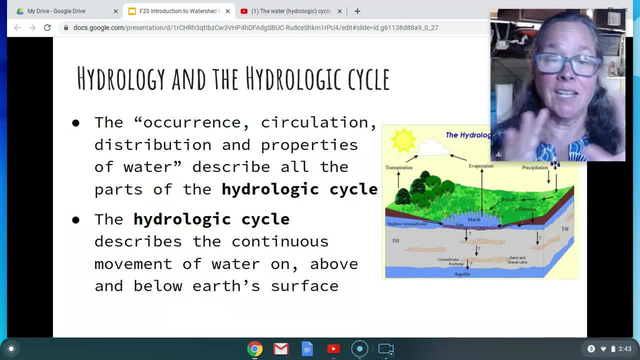 Overall, the hydrologic cycle is this continuous movement, describing the continuous movement of water on and below the earth. So that's something to really think about. A lot of times we think about just what we can see, but there's a lot of underwater water that's underground that we can't see. that's moving. 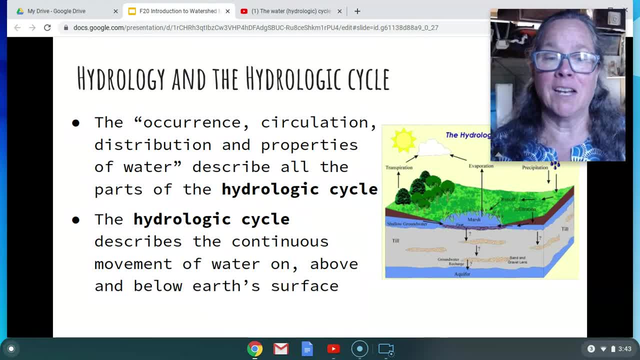 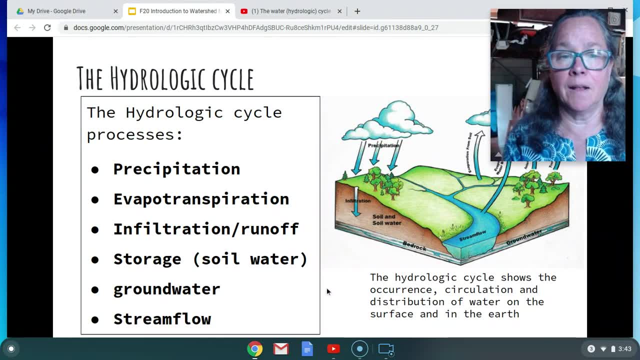 and that we need to consider in whenever we make management decisions. so we'll be. we'll be talking about that. So here are some of the processes, and this pretty much outlines a lot of this course, because we're going to start talking about precipitation. Then we're gonna look at the process of water loss and what happens when we make decisions about that, and then we're gonna look at the process of water loss and how we can bring it down. We're going to look at the process of water loss and how we can bring it down. 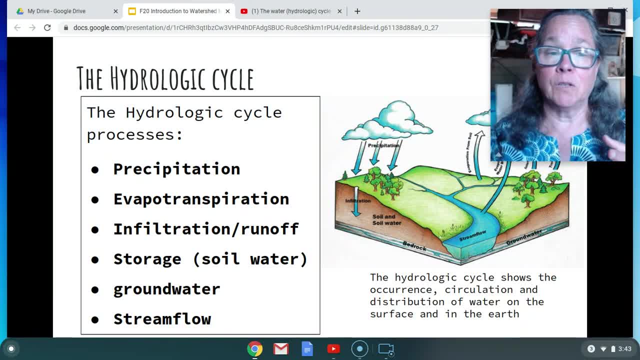 How we're moving a lot- Let's just watch this for a second- at evapotranspiration, infiltration, runoff, storage, groundwater and streamflow. So you'll become very familiar with all of these processes- and you might already be familiar with them- and 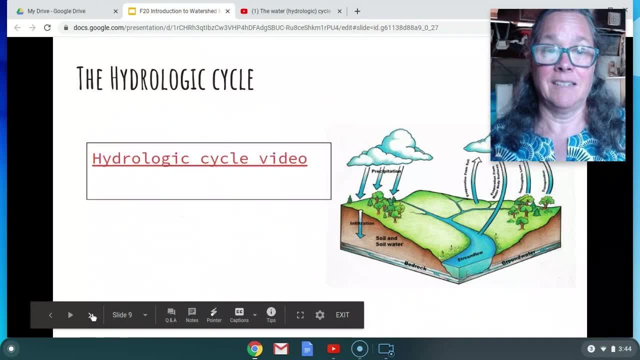 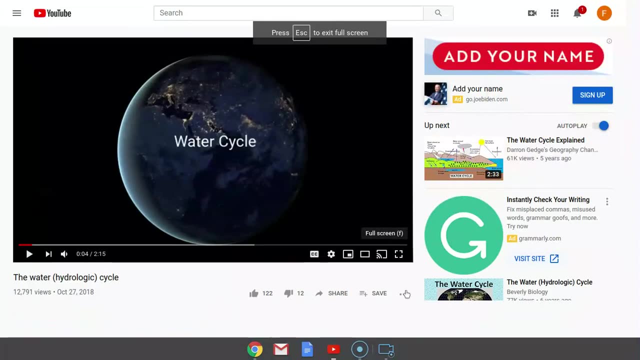 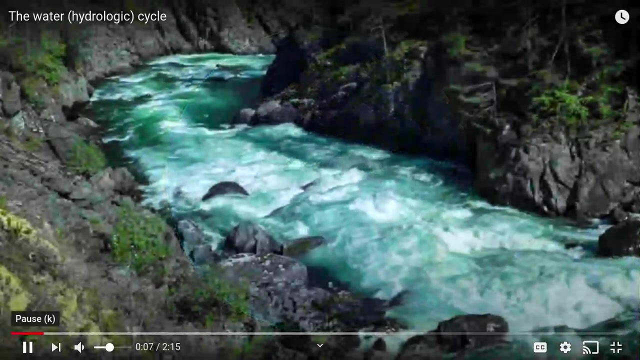 that's great. I'd like to share with you a little video now about the hydrologic cycle, just to give you a review. perhaps- and we'll- we'll be talking about again in a lot more detail. So let's look at this. Let me get this up and running. The water we use today has been around for a long, long time. 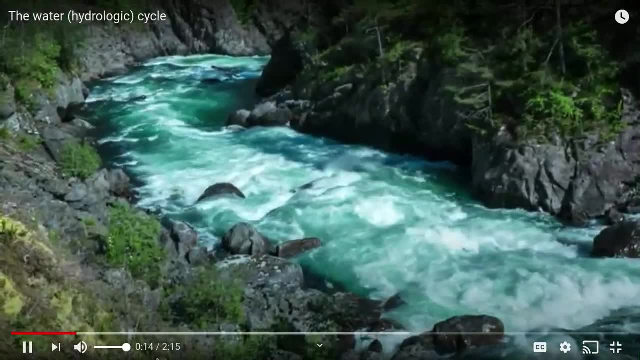 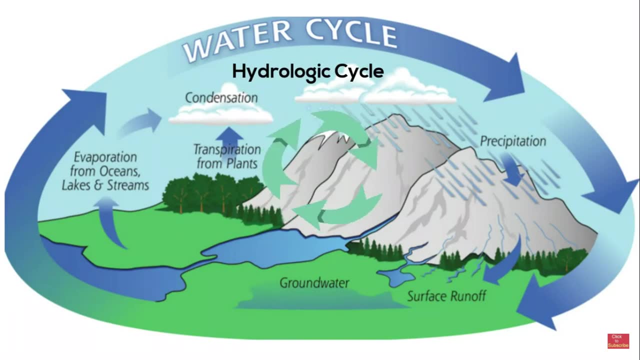 That is because water can recycle itself in the water cycle, which is also called the hydrologic cycle. Let's start this cycle with the evaporation of water. So the water cycle is a cycle of water that is being recycled from the surface of the ocean. 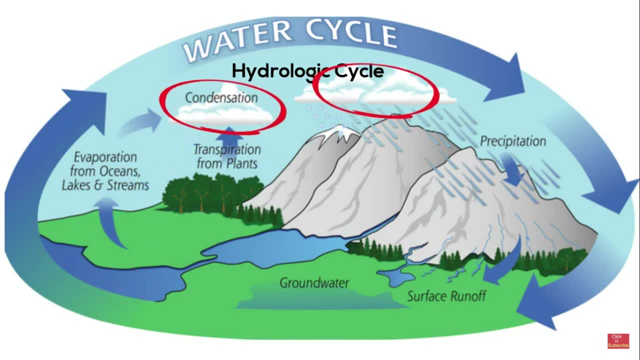 As this moist air is lifted, it cools and water vapor condenses. It may form clouds. In fact, clouds are made up of tiny water droplets and ice crystals that are so small they can float in the air. This moisture in the atmosphere may be transported around the globe until it returns to. 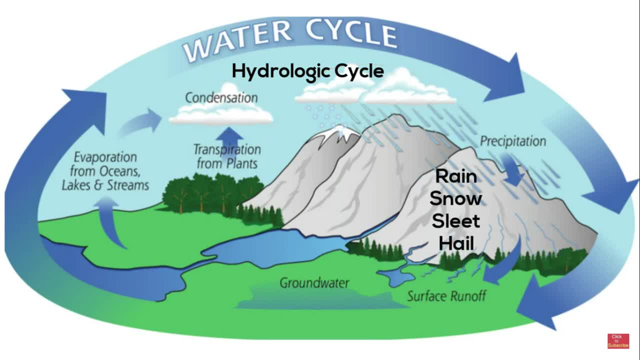 the surface as precipitation. It may take the form of rain, snow, sleet or hail. Now, once this water reaches the ground, one or two processes may occur. Some of the water may evaporate back into the atmosphere, or the water may penetrate the surface and become groundwater. The groundwater may take several 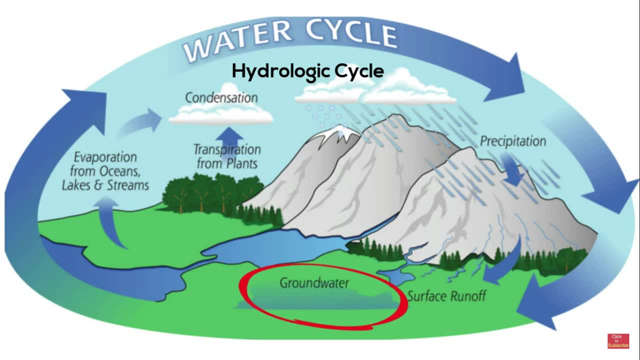 different paths. The groundwater may seep in its way into the oceans, river or streams, Or it may go into an aquifer, which is a body of saturated rock through which water can easily move, Or it may be released back into the atmosphere through transpiration. Transpiration occurs when 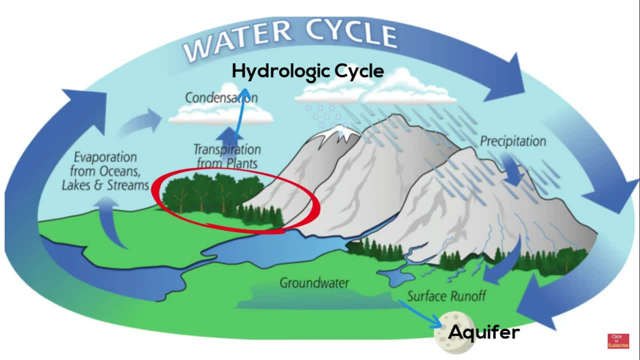 leaves from trees and other vegetation give off water vapor through pores in their leaves. Some water on the earth's surface is not absorbed by plants or become groundwater and it becomes surface runoff. This runoff may empty into lakes, rivers and streams and then is carried. 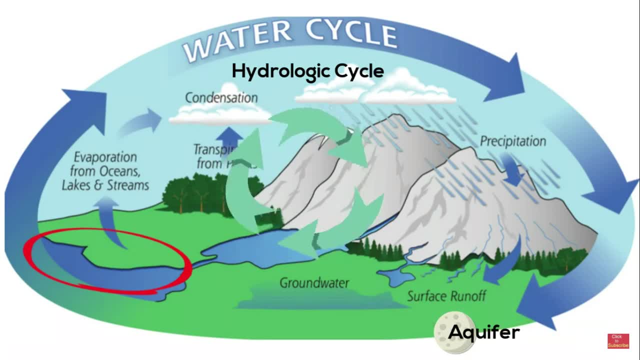 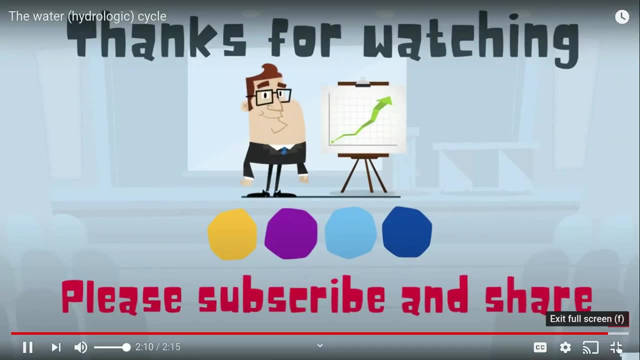 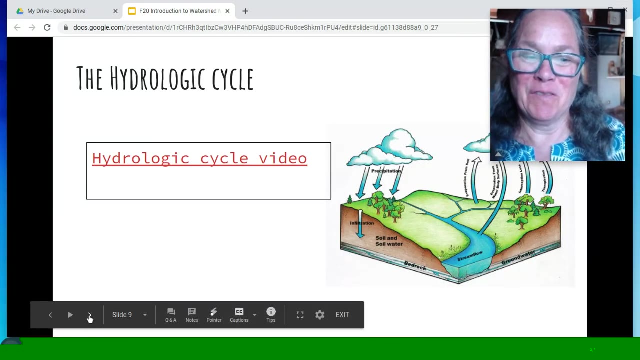 back to the ocean, where the cycle may begin. So there we go: the basics of the water cycle. Thanks for watching, and MooMooMath uploads a new math and science video every day. Please subscribe and Okay, that's your overview. Be prepared to get a lot more detail in that. 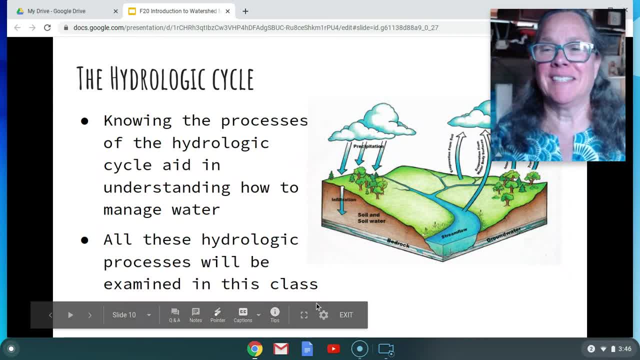 As we move on in this semester. So knowing these processes of the hydrologic cycle are going to really aid your understanding of how to manage water. And I want you to keep that perspective, because we are going to get into a lot of detail And if you just consider that, 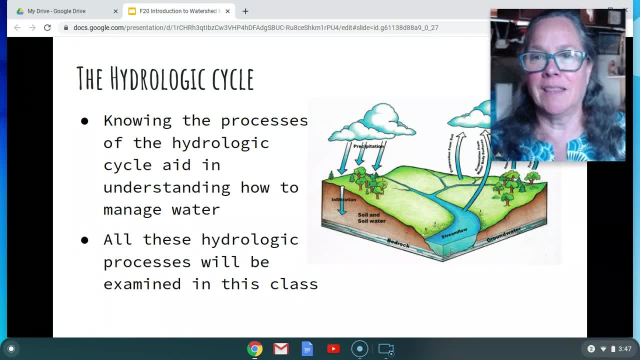 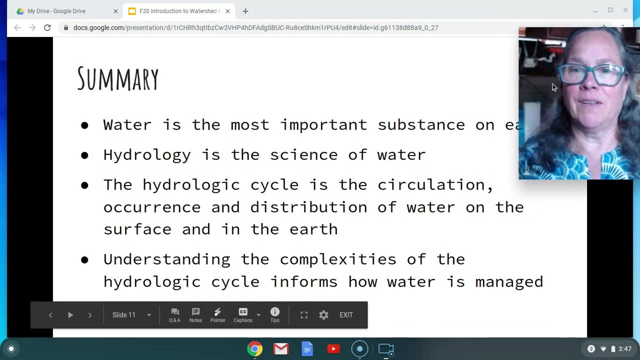 knowing these things is going to help with the management of water, And I think the reading material I have for you also will help emphasize that. So get ready, Let's just summarize what I've talked about so far And I'll move myself out of the way. 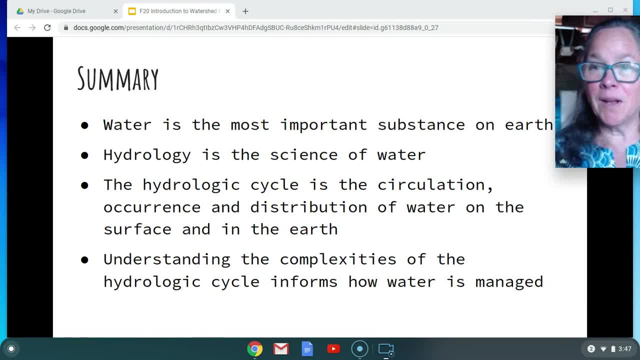 a little bit here. Water is the most important substance on earth And hydrology is the science of water. The hydrologic cycle is the circulation, occurrence and distribution of water on the surface and in the earth. So I kind of added that a little bit just to emphasize that. So understanding.